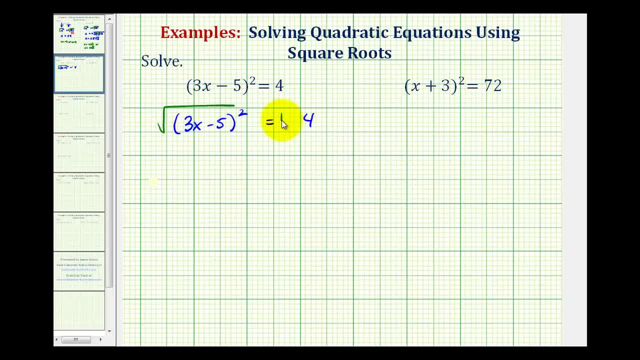 So the square root of the left side must equal, plus or minus the square root of four. Well, looking at the left side of this equation, since we have two equal factors underneath the square root, this is a perfect square. so it's going to simplify to just one factor of three x minus five. 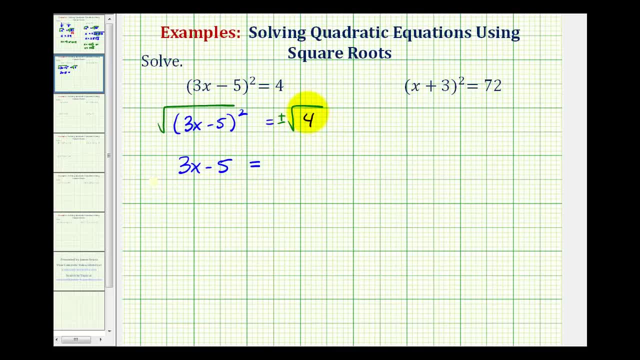 Now on the right side, since the square root of four is equal to two, we have plus or minus two, And now we can just solve this for x to determine our two solutions. So for the next step, we'll add five to both sides of the equation. 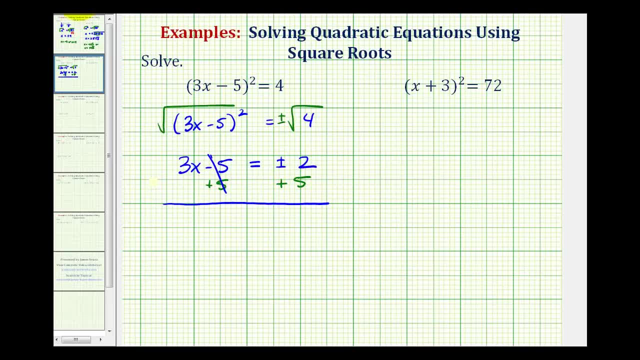 Minus five plus five is zero. That's why we did that. So now we have three x equals. on the right side, we have five plus or minus two. Leave this in its current form for right now. The last step here is to divide both sides by three. 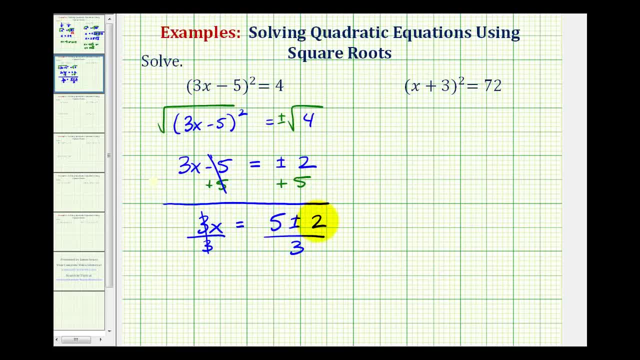 So this gives us x equals five plus or minus two divided by three. Now, we don't want to leave it in this form. We actually want to determine the two solutions. So one solution is x equals five plus two divided by three, And the other solution is x equals five minus two divided by three. 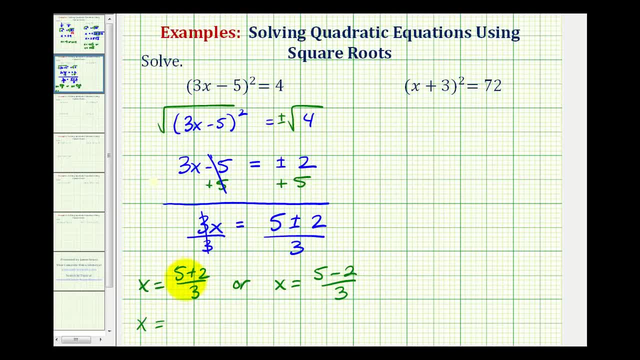 Let's go ahead and simplify these. So here we have: five plus two is seven, so we have seven thirds or x equals over here. five minus two is three. Three divided by three is equal to one. So our two solutions are: x equals seven thirds or x equals positive one. 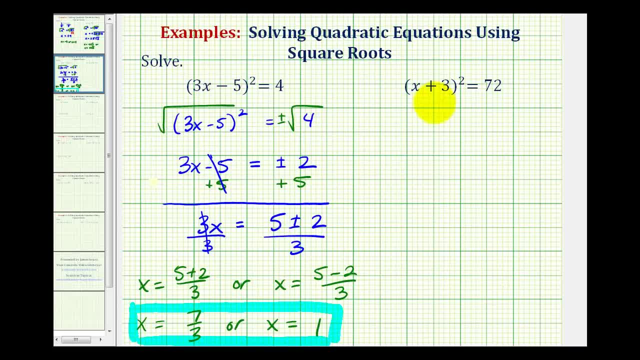 We're going to use the same technique in our second example. For our second example, we'll apply the same technique Again. notice how the left side of the equation, which contains the variable x, is a perfect square. So we can undo the squaring by square rooting both sides of the equation. 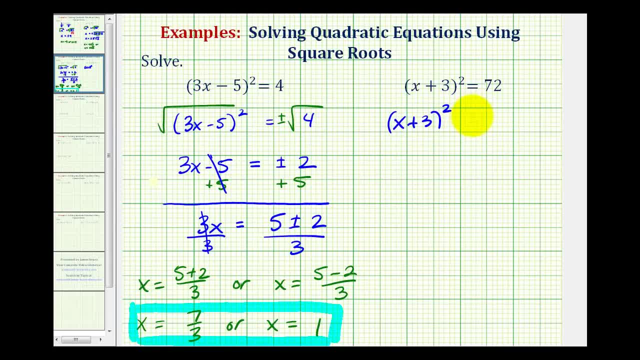 So we have: the quantity x plus three squared equals seventy-two. So now we'll square root both sides. Remember, we have a plus or minus here to obtain our two solutions. The quantity x plus three squared is a perfect square. So the left side simplifies to one factor of x plus three. 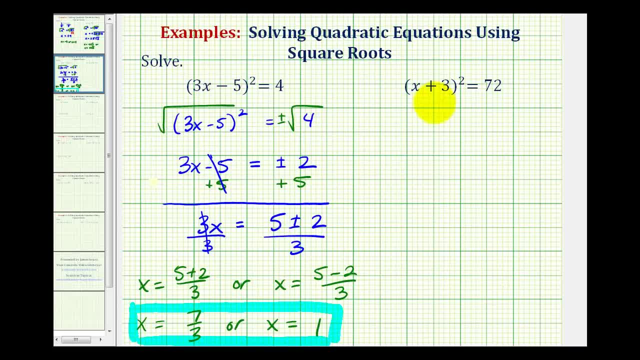 We're going to use the same technique in our second example. For our second example, we'll apply the same technique Again. notice how the left side of the equation, which contains the variable x, is a perfect square. So we can undo the squaring by square rooting both sides of the equation. 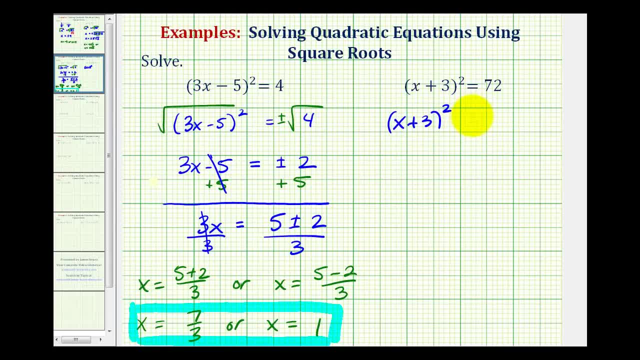 So we have: the quantity x plus three squared equals seventy-two. So now we'll square root both sides. Remember, we have a plus or minus here to obtain our two solutions. The quantity x plus three squared is a perfect square. So the left side simplifies to one factor of x plus three. 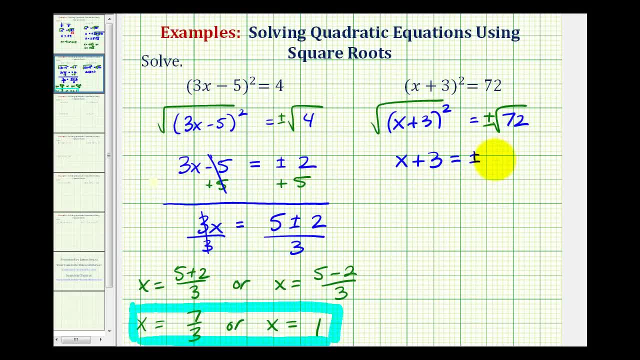 On the right side we have plus or minus the square root of seventy-two. Notice, seventy-two is not a perfect square, but it does contain perfect square factors, Since seventy-two is equal to thirty-six times two and the square root of thirty-six would be six. 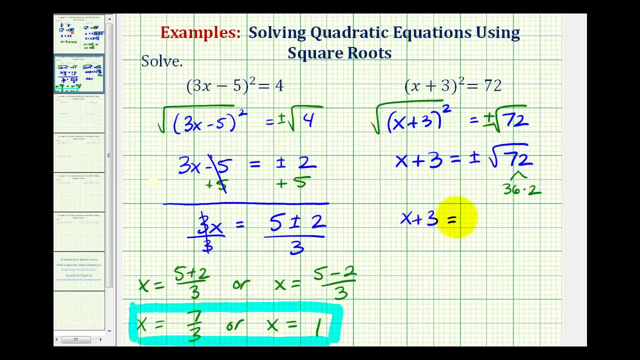 this simplifies to the quantity: x plus three equals plus or minus six. square root two. If I lost you there, remember the square root of seventy-two can be written as the square root of thirty-six times two And again, the square root of thirty-six is six. 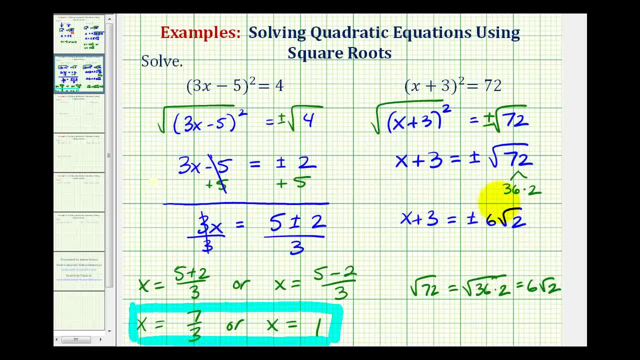 and the two stays underneath the square root. So that's where this came from. And for the last step, we just need to subtract three from both sides of the equation. This would be zero. So we have x equals. I need to be careful here, because these are not like terms. 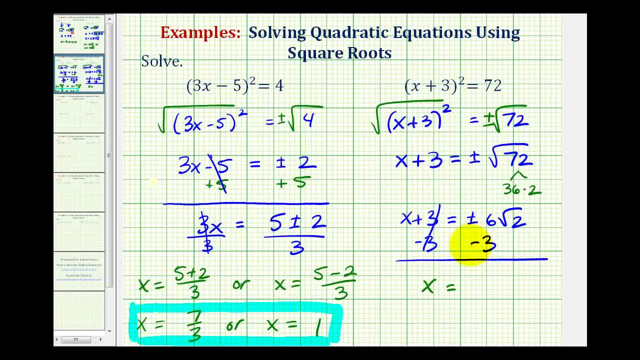 This contains a radical and this doesn't, So our solution is just negative three plus or minus six square root two. If we wanted to list the two solutions, we would have x equals negative three plus six square root two, or x equals negative three minus six square root two. 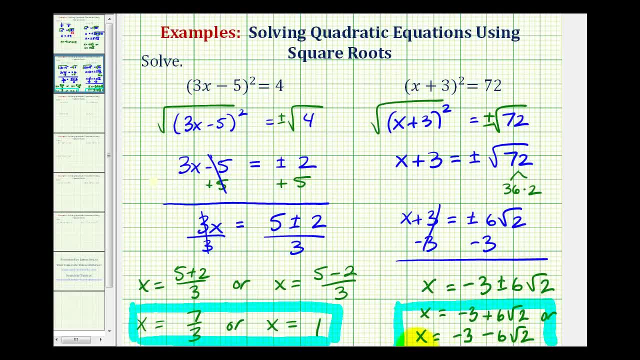 These do not simplify any further. Okay, I hope you found this helpful. Thank you for watching.